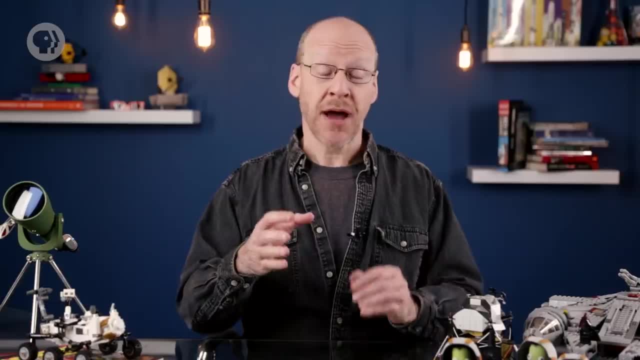 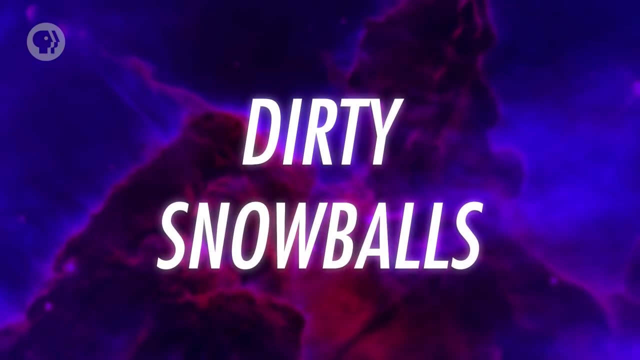 ammonia, things we normally think of as gases on Earth, And by rock I do mean rocks, but also gravel and dust. In fact, astronomers sometimes call comets dirty snowballs, Which isn't a half-bad term. It's that ice that makes comets well comets. When they're way out in deep space they're so cold that they're basically inert lumps of ice and rock. But many are on elliptical orbits that take them from those sub-freezing depths into our neck of the woods where the Sun can warm them As they heat up the ice. 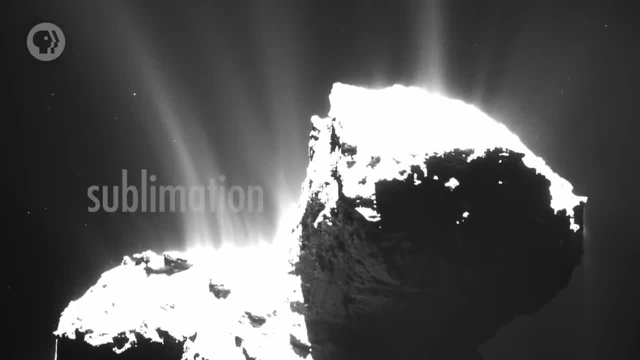 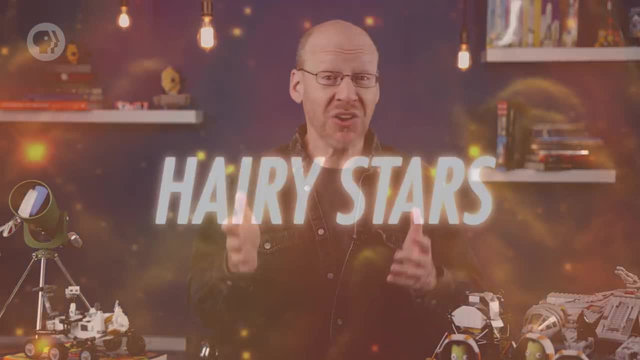 turns directly into a gas, a process called sublimation. The gas then flows away from the comet, creating a cloud around it. This makes the comet look fuzzy, and actually in the past they've been called hairy stars. I like that term too, and in a sense we still use it. The solid part of the comet is called the nucleus and the gaseous cloud around it is called the coma- Latin for hair. In fact, that's why we call them comets. As the ice sublimates, the bits of rock and gravel and dust embedded in it can be freed. 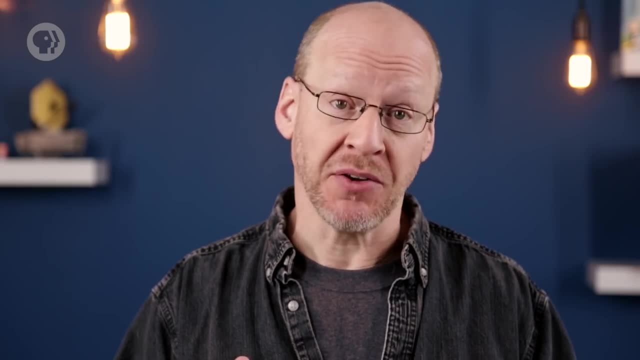 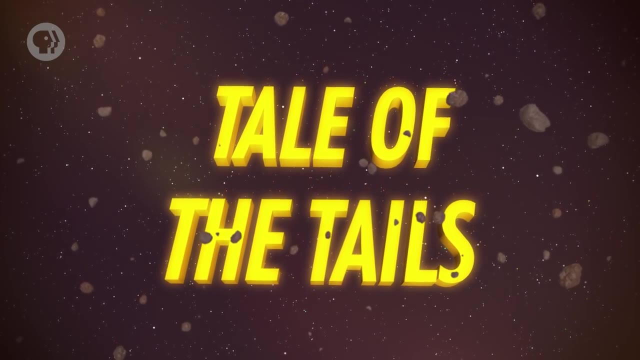 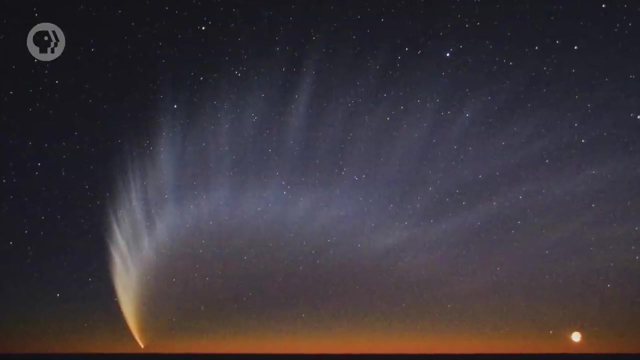 and leave the nucleus as well. This material is what forms the comet's tail, but how that happens depends on which material you're talking about. The gas and the dust from comets form two different tails. Gas molecules emitted by the comet get ionized by the Sun's ultraviolet light. That means they lose electrons, becoming 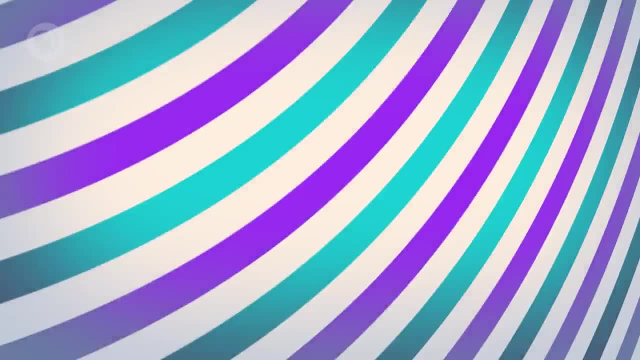 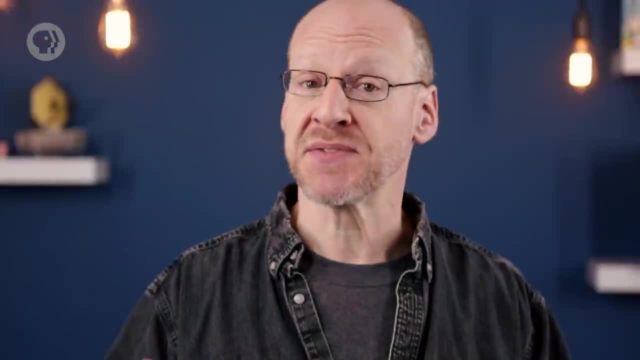 charged and charged particles are highly susceptible to magnetic fields. The solar wind is a stream of charged particles blown out by the Sun and carries a magnetic field with it. As the wind hits the ionized gas from the comet, it picks up those particles. 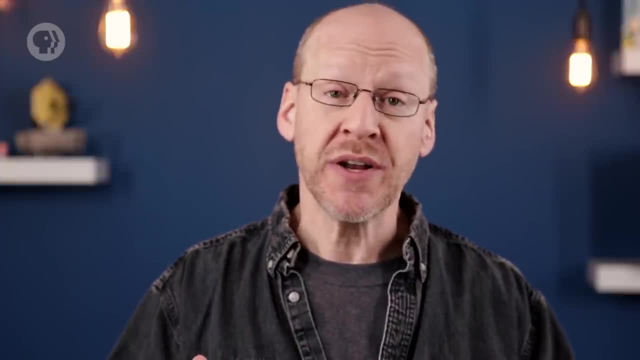 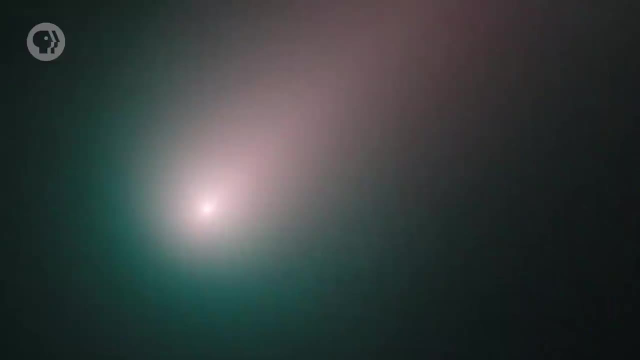 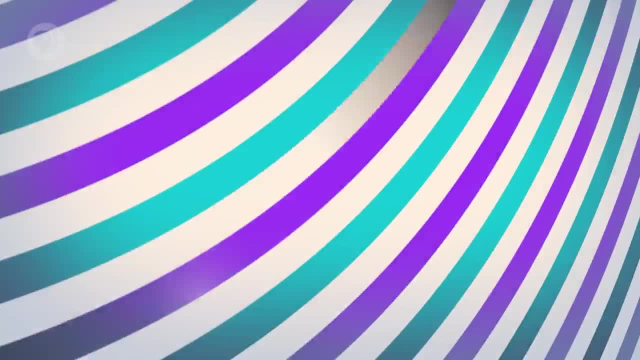 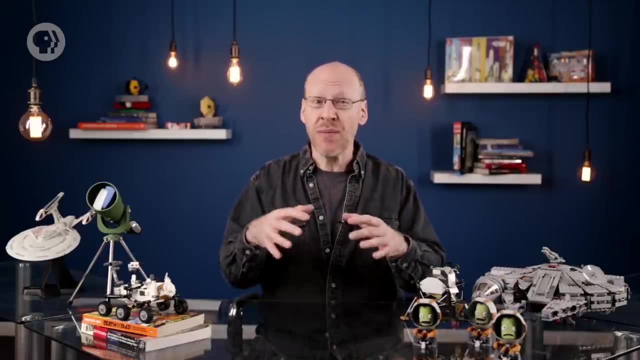 sunlight. Light from the Sun exerts a small but inexorable pressure, and this pushes on the dust particles. The dust streams away, but because the pressure isn't as intense as the solar wind is on the gas tail, the dust tail blows away more lazily and tends 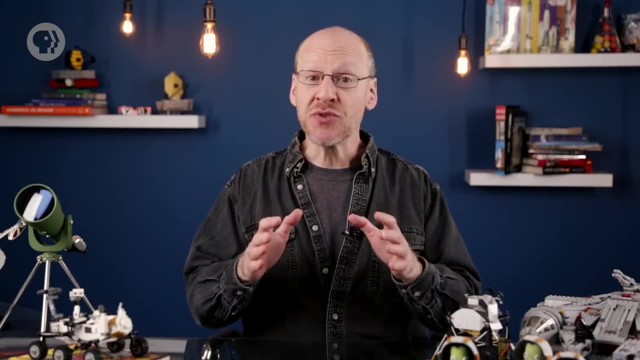 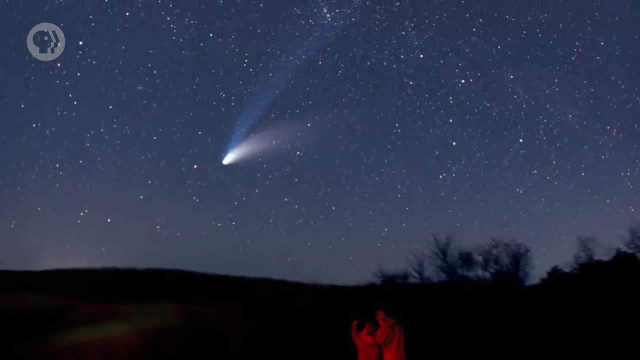 to lag behind the comet in its orbit. That means the two tails usually point in two different directions. In some comets, like 1997's incredibly bright and gorgeous comet Hale-Bopp, this is pretty obvious. The dust tails look white or a teeny bit yellowish due to reflected sunlight. 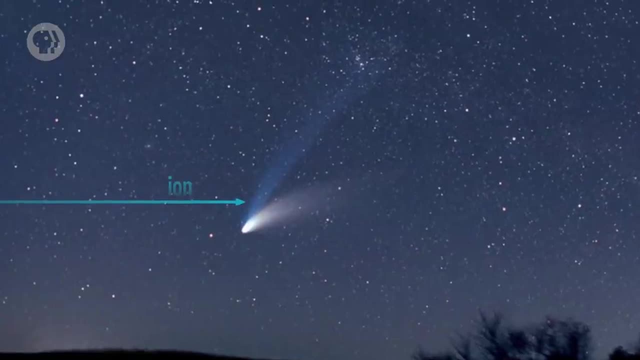 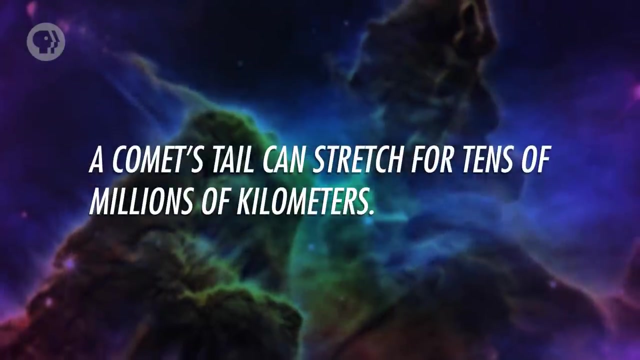 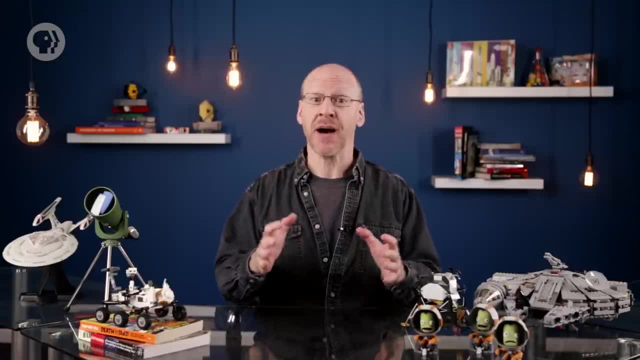 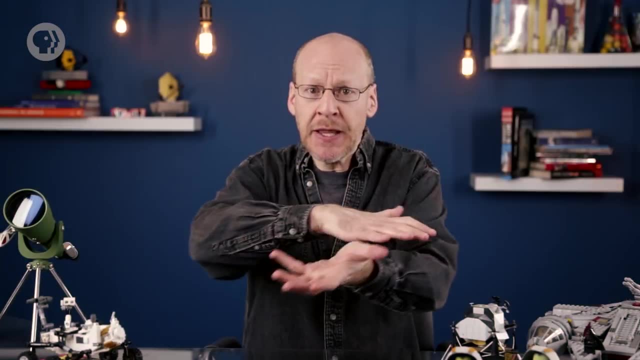 isn't that big of a problem. Broadly speaking, comets are classified by their orbits. If they have orbital periods less than 200 years, they're called short-period comets. These tend to orbit the Sun in the same plane as the planets and go around the Sun in the same direction as well From Earth. we see them sticking near the ecliptic, the line across the sky that marks the annual path of the Sun. Comets that take longer than two centuries to go around the Sun are called long-term comets and have orbits that are tilted every which way. That means they can. 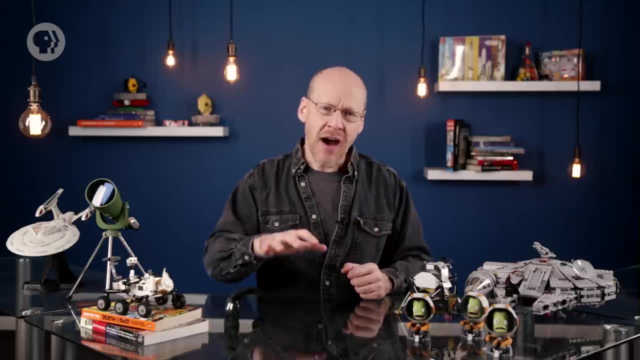 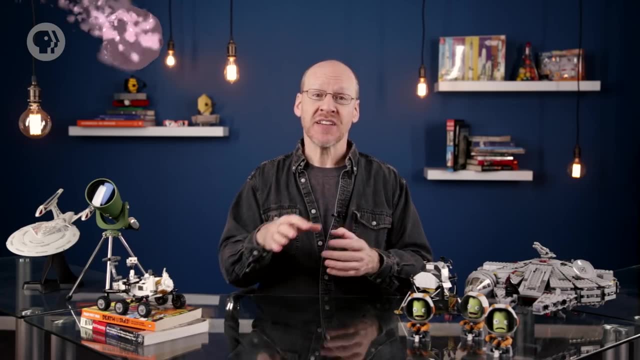 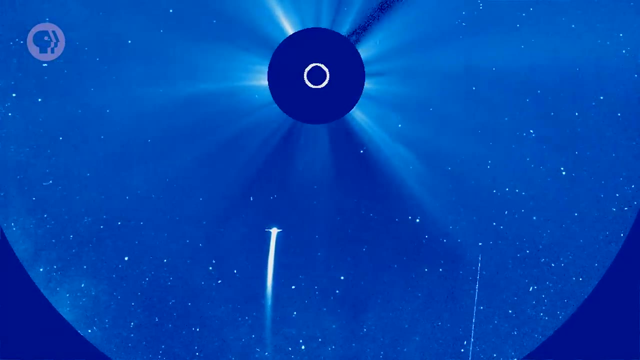 appear anywhere in the sky. But this raises an interesting point. Comets go away Every time they get near the Sun and start outgassing. they lose mass Over time. they get smaller. Eventually they should evaporate. Some do this all at once because they dive into the Sun, skimming our star's surface. 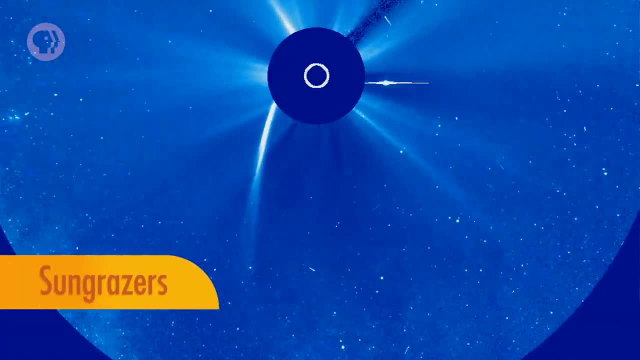 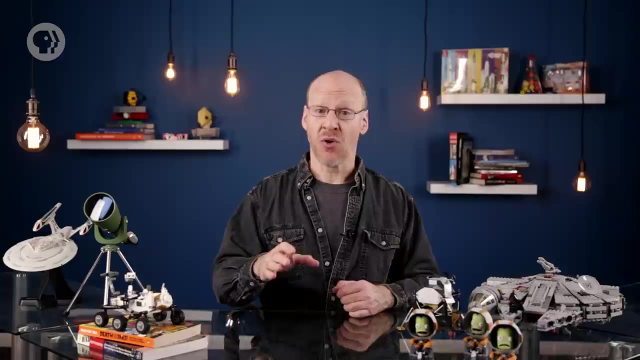 We call those sun divers or sun grazers. Many of those may actually be pieces from a bigger comet that broke up in space nearly a thousand years ago. But besides those, we know of some comets with orbits that can be short, some with periods. 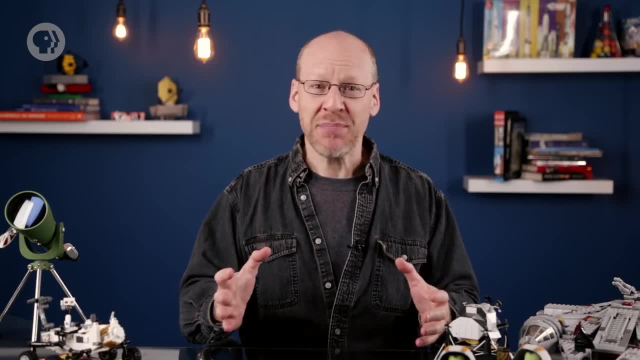 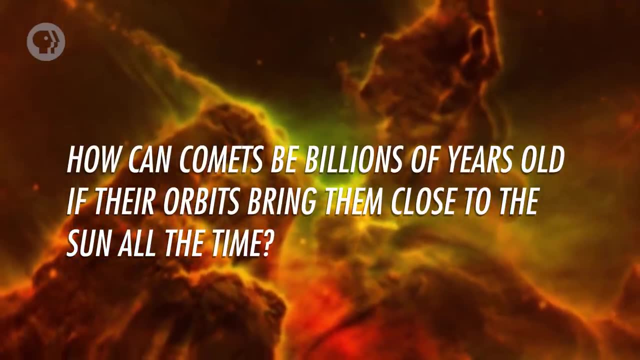 of just a few years. Even a century is like a single flap of a mosquito's wing compared to the lifetime of the solar system. How can comets be billions of years old if their orbits bring them close to the Sun all the time? 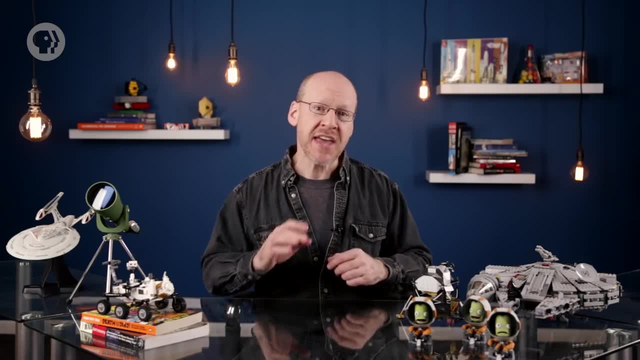 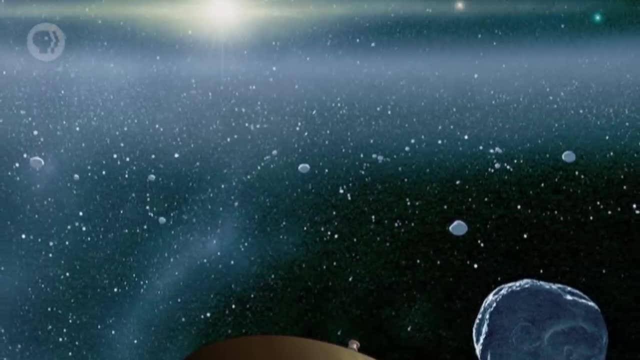 Ah, astronomers wondered about this very thing. Over the years, they came up with an idea: Maybe out past Neptune there's a repository of comets, Chunks of dirty ice, Millions of them, Billions, Orbiting the Sun. where it's perpetually cold. They could have orbits that last for millennia or more, But then something tweaks them, makes them fall toward the Sun. In fact, there may be two such regions, since we have both short-period and long-term comets. 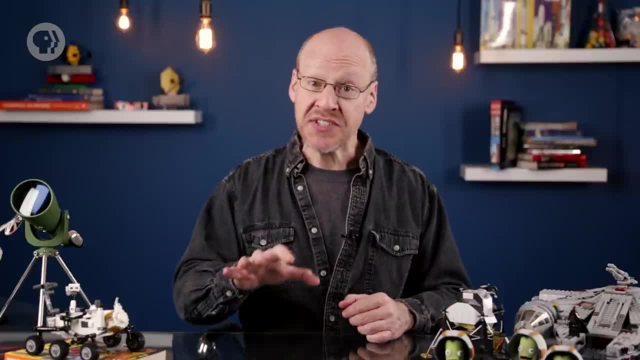 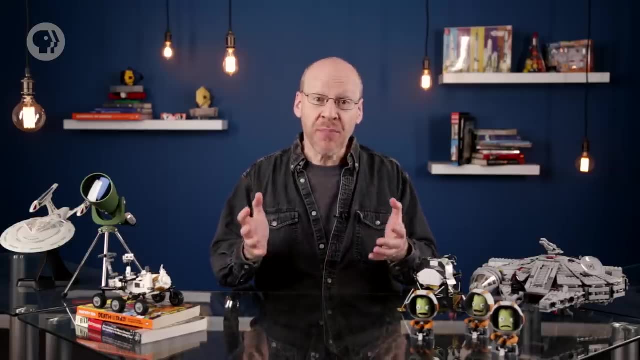 Turns out, this idea is correct. We now know enough about those distant regions of the solar system that they deserve their own episode, so we'll dive into that topic later. So what do comets? look like up close, Like really close. 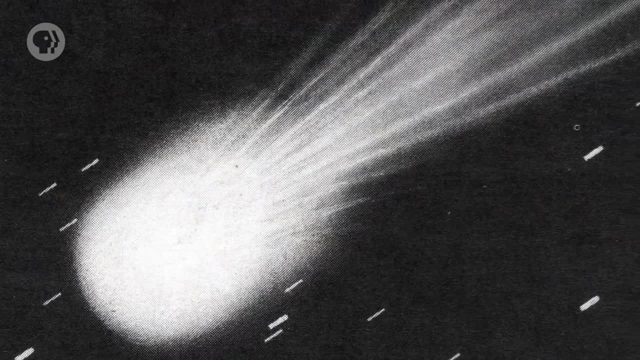 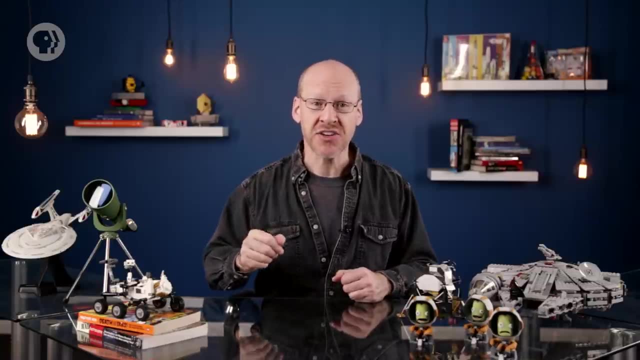 Studying them from Earth is hard. The coma obscures the nucleus, making it nearly impossible to see it directly. Ah, from Earth. If you instead send your telescope to a comet, things change. We first did that in the 1980s, the last time Comet Halley came around. Several nations sent spacecraft to 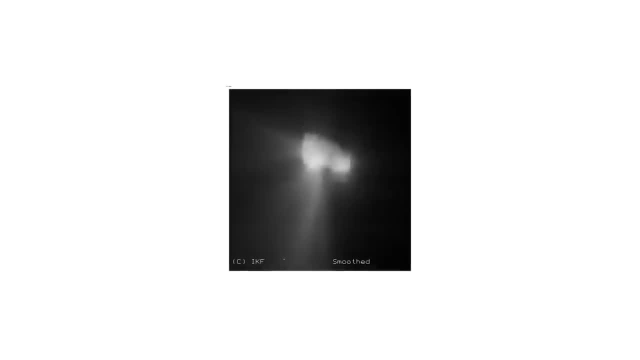 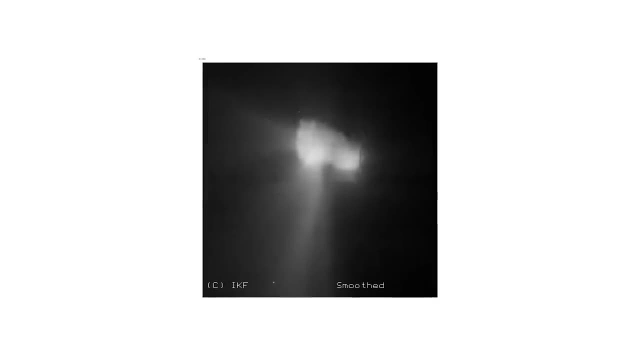 fly past the comet, and the Soviet mission Vega 1 was the first to successfully get pictures of the nucleus. The low-resolution images revealed a dark lump, highlighted with two bright spots, later determined to be jets of gas streaming away. These images were used to better determine. 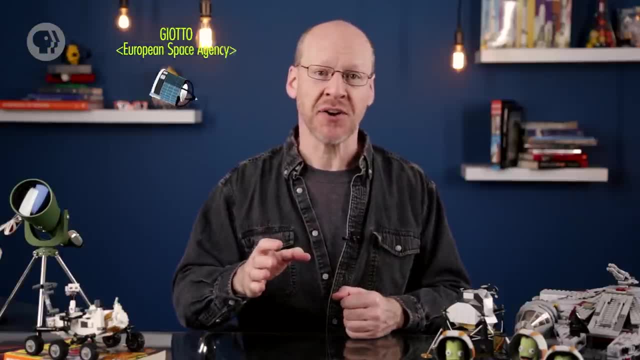 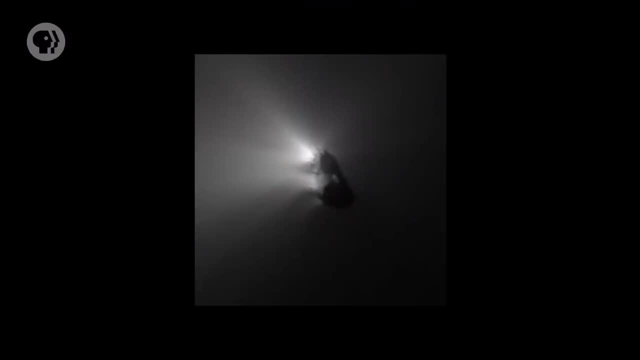 the position of the nucleus and a few days later the European probe Giotto zipped past the nucleus at an incredibly close distance of just 600 kilometers. Those pictures were more detailed and showed us a flying mountain in a regular chunk, 15 by 8 kilometers in size. 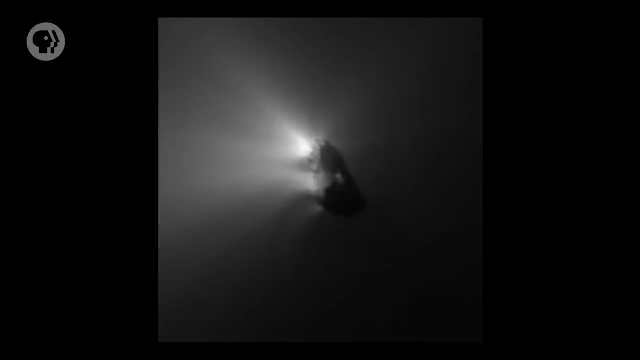 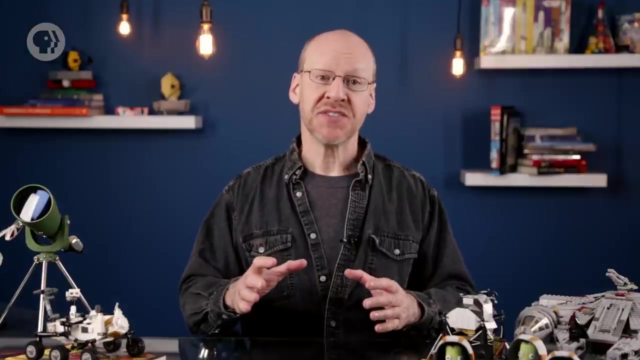 And it was dark, reflecting only 4% of the light that hit it. That makes the nucleus as black as asphalt. You might think that all that ice would be shiny, but it's not that simple. Most of Halley's nucleus is covered in thick dust laced with darker molecules, with only 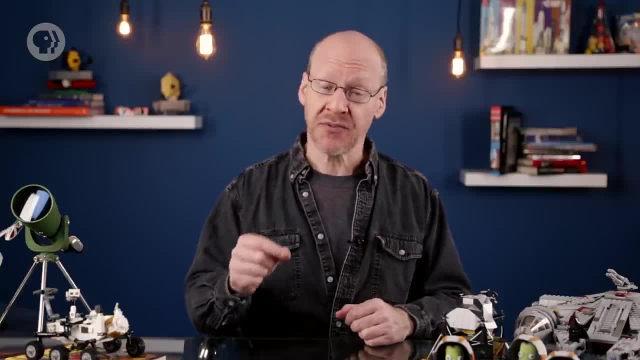 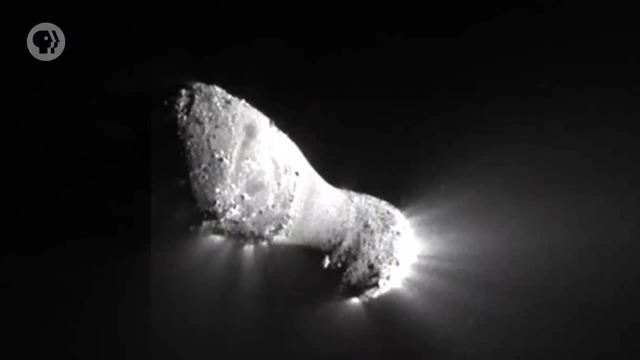 a few spots emitting gas. Most likely there are deposits of ice under the surface and only some of them receive enough heat from the Sun to sublimate and blow out gas. This has been seen with other comets as well. The gas is emitted from specific spots on. 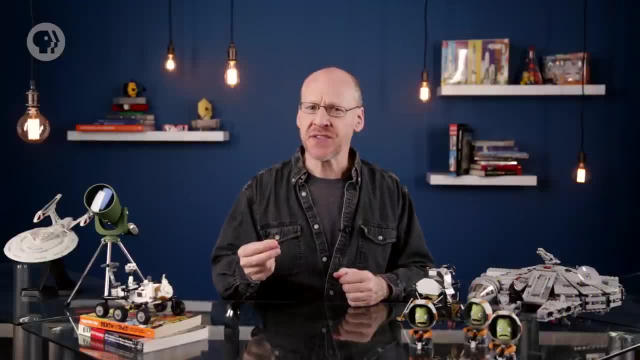 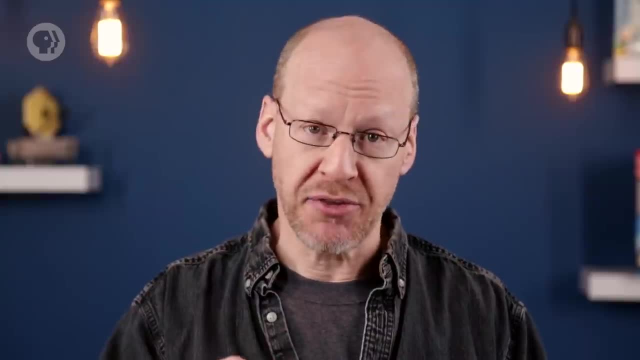 the comet venting out from cracks in the crusty surface. The surfaces of comets must be inhomogeneous, different in different places. That fact was brought home magnificently in 2014 by another European mission, Rosetta. It went into orbit around the comet 67P Churyumov-Gerasimenko and found its orbit in the Comet 67P Churyumov-Gerasimenko. 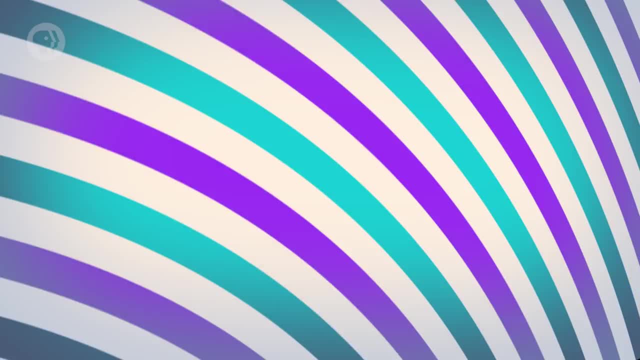 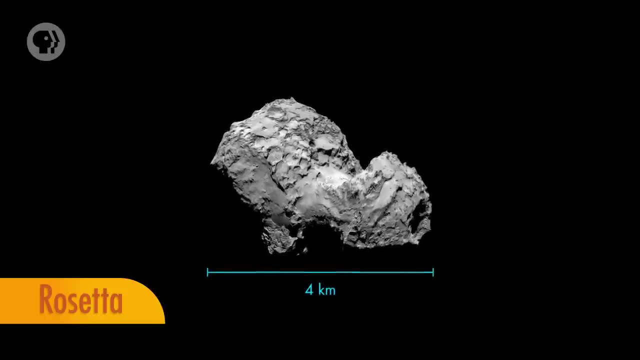 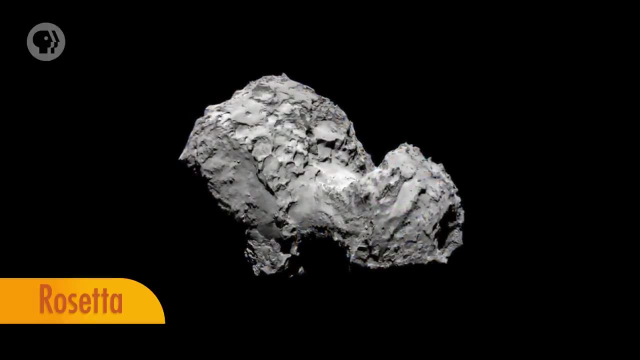 Measuring about 4 kilometers end to end. 67P has two lobes connected by a narrow neck looking very much like a cosmic rubber ducky. The surface is completely devoid of craters. Clearly the surface is very young. Images show jets of gas emitted from very specific 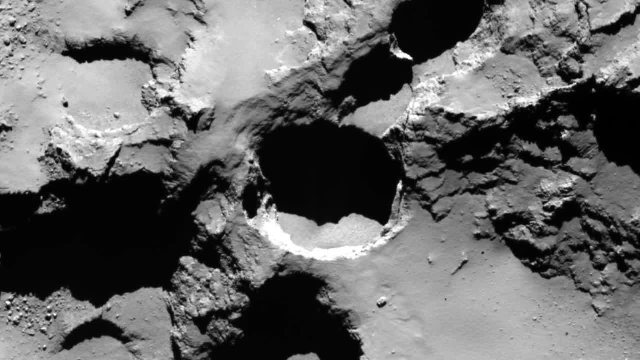 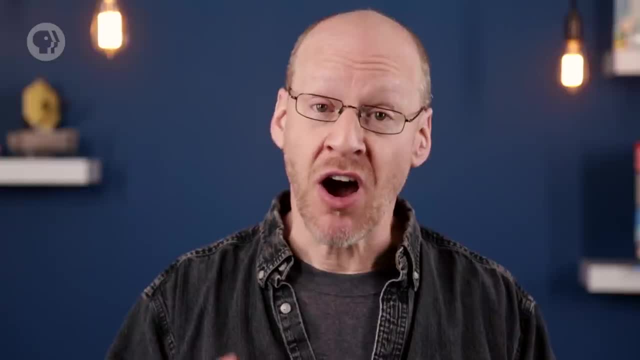 places on the surface and there are wide circular pits here and there which may be gas vents growing wider over time as the ice below is depleted. Surprisingly, the surface is fairly tough and hard, And some scientists expected it to be fluffier. 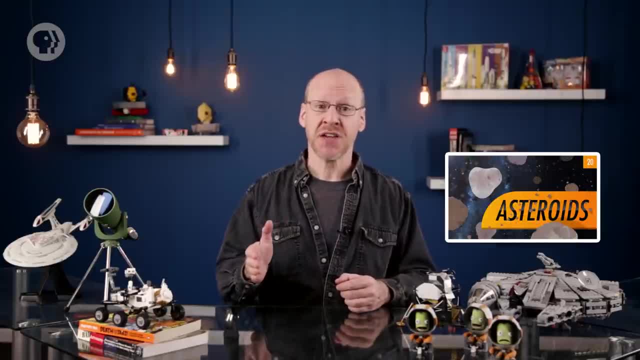 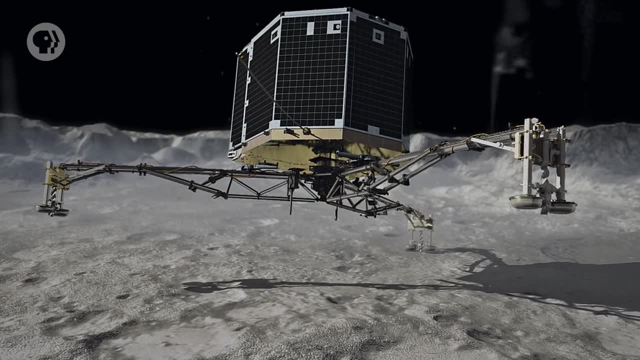 The comet has a very low density, similar to rubble pile asteroids, so it was expected that the surface would be soft. Rosetta sent down a lander named Philae to set down on the surface using harpoons to anchor itself, But instead the lander bounced, unable to penetrate the tougher than expected material. One idea to explain this is that the ice is porous and fluffier inside the comet, but as it nears the Sun, the ice at the surface warms and changes its structure, forming that harder crust. As for the double lobe thing, well, that's a bit baffling. We see some asteroids shaped. 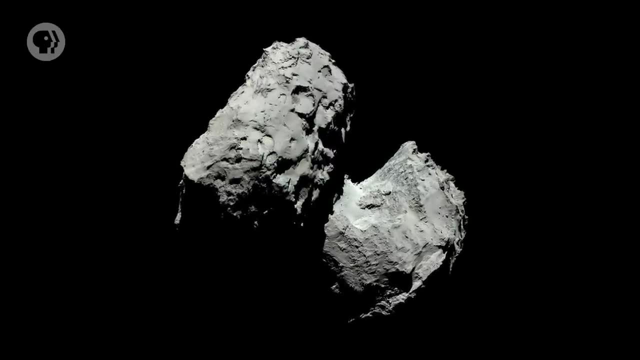 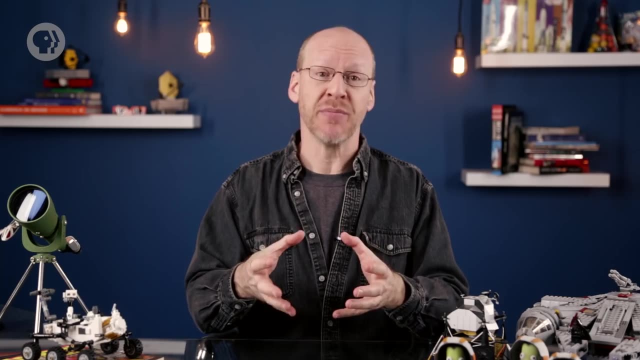 that way as well, It's possible. 67P used to be two separate comets that had a low-speed collision and stuck together. Or maybe it used to be one big lump, but over the eons the ice in the middle sublimated more, leaving behind the two lobes. 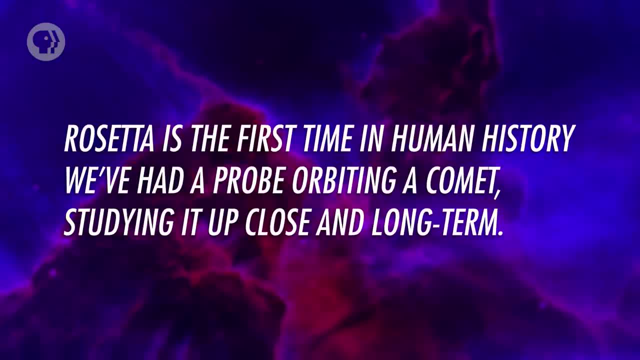 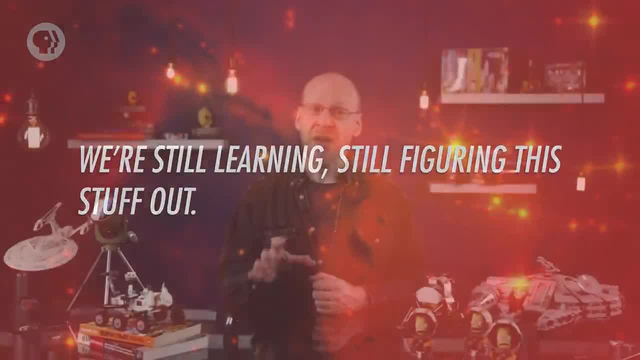 Rosetta is the first time in human history we've had a probe orbiting a comet, studying it up close and long-term. We're still learning, still figuring this stuff out. Incidentally, I mentioned earlier that A Comets have a long-term relationship with the Sun and B Comets have a long-term relationship. with the Earth Comets have lots of ice in them and two, they also get really close to Earth, sometimes, In fact, they can hit us. Now, not to get all technical and scientific-y, but that is what we would call bad, as we'll discuss in an upcoming episode. 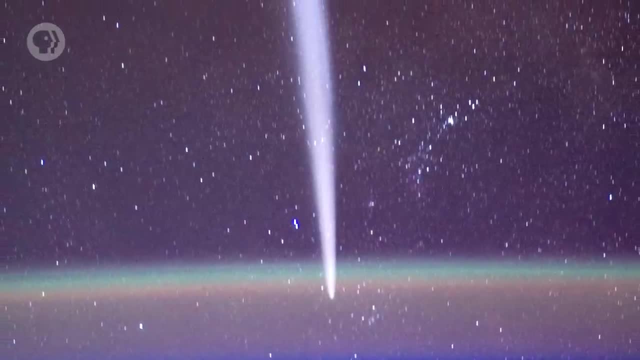 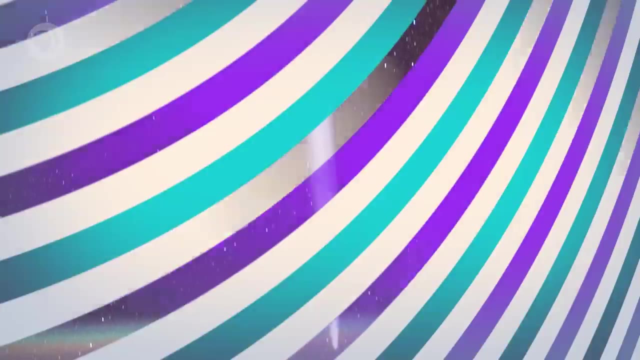 But billions of years ago, lots of comets hit the Earth, not long after our planet formed, Together with asteroids, many of which are also rich in water ice. they may have brought a significant amount of water to Earth. Scientists are still wrestling over the details of this. 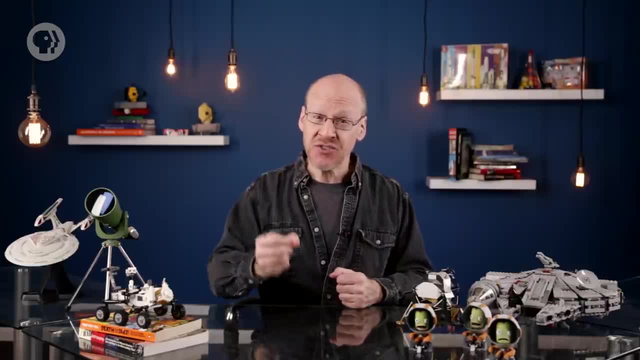 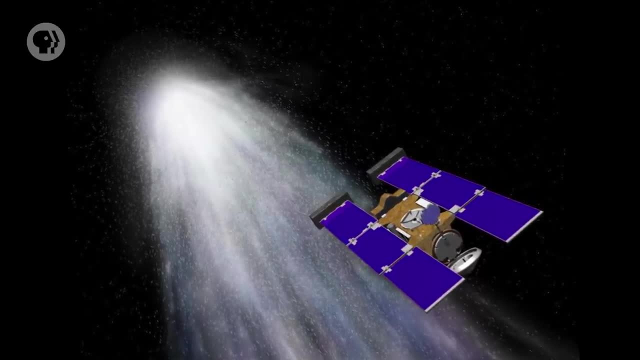 and it may be a while before the actual numbers are nailed down, But it's an intriguing thought. Even more interesting In 2004, NASA's Stardust space probe physically passed through the coma of Comet Vilt 2, collecting samples that were returned to Earth. Careful analysis of 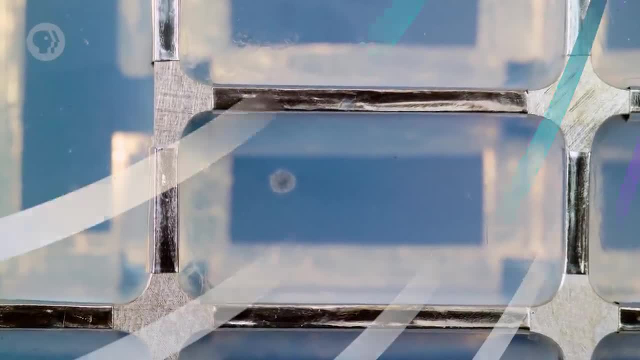 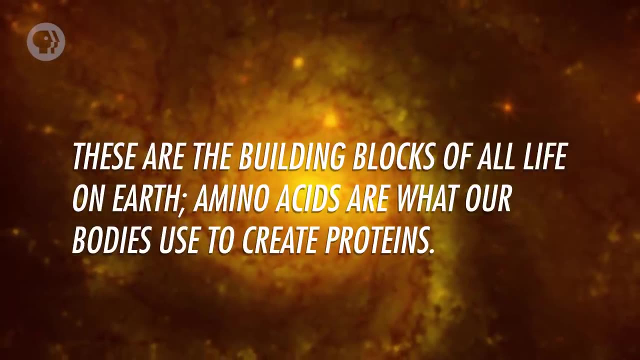 the material found the presence of organic carbon-based molecules in them, And not just any random molecules, but complex ones, including amino acids. These are the building blocks of all life on Earth. Amino acids are what our bodies use to create proteins. 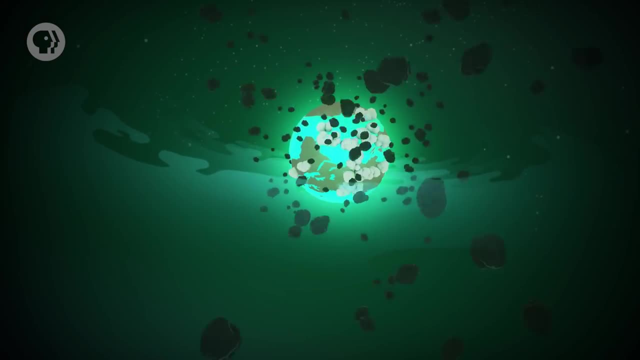 It's possible that the ingredients of life on Earth didn't start here but in the past. But it's possible that the ingredients of life on Earth didn't start here but in the past, But instead were brought to our planet from comet impacts, Or at least there was a mix. 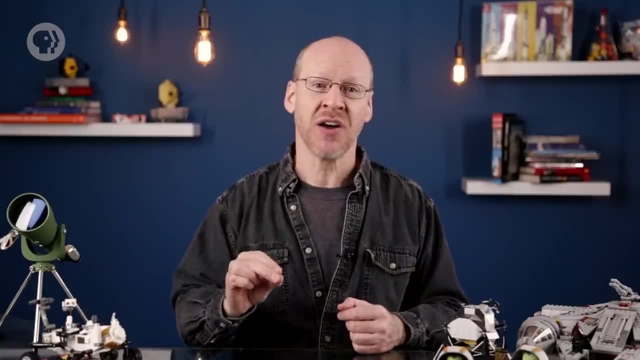 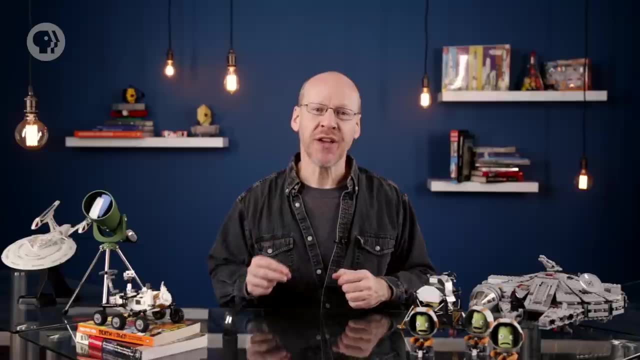 of the two. If that's the case, then in a sense all life on Earth is part alien. How about that? But what gets me are the philosophical ramifications of this. When we look into space, when we examine our celestial neighbors, when we send probes to comets and survey what we find, 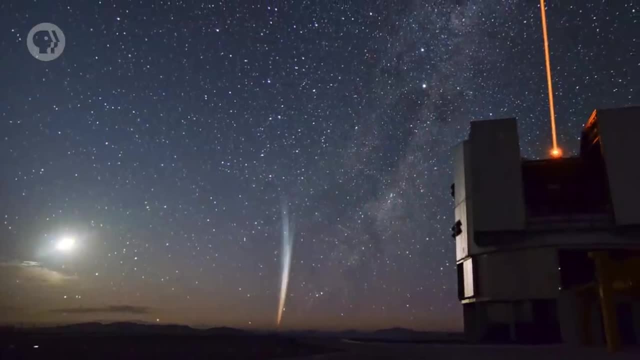 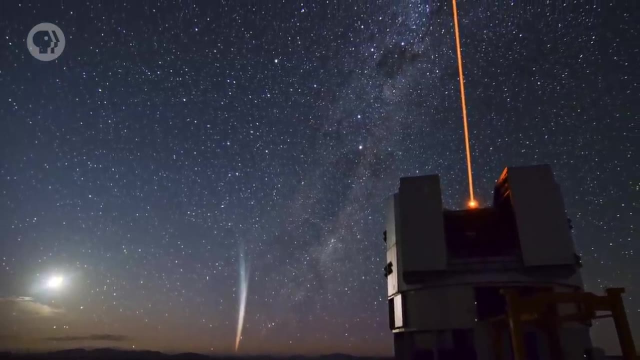 we're looking at our own origins. Comets are like time machines, allowing us to investigate our past four billion years back, Hinting at the secrets of the origin of life itself. And you thought astronomy was just lying out in a field and looking up. Well, it is, but